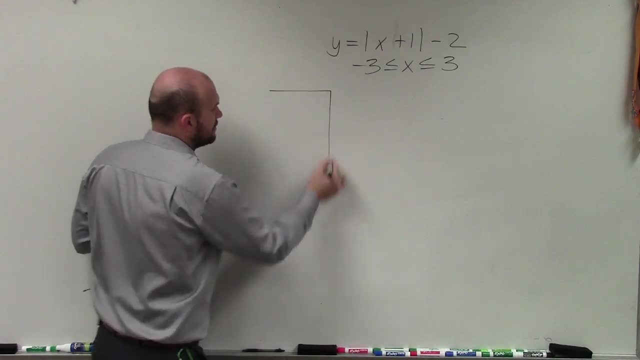 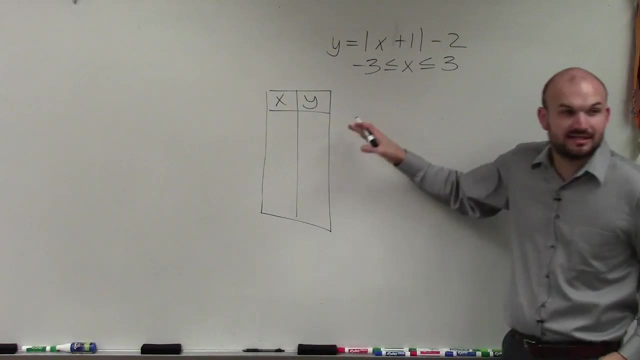 So to create a table of values, all we're simply going to do is we're going to have x coordinates and we're going to have y coordinates And, as my constraint states, I want values of x between negative 3 and 3.. 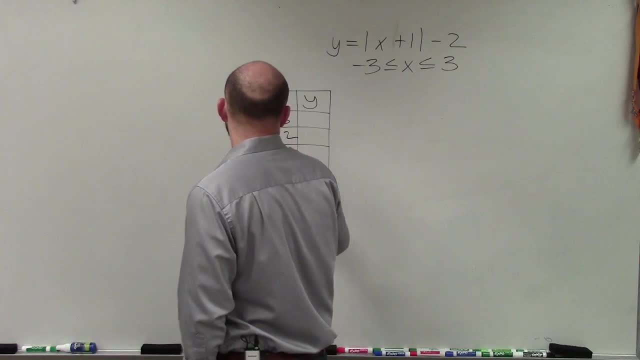 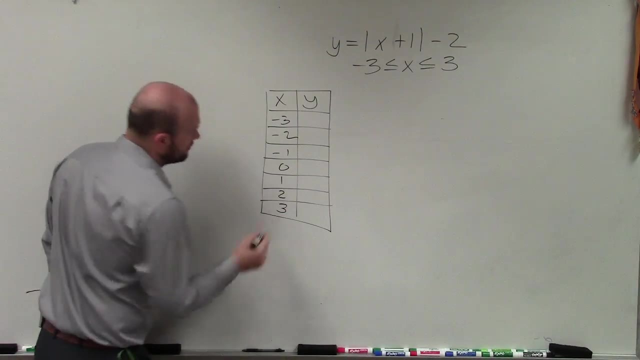 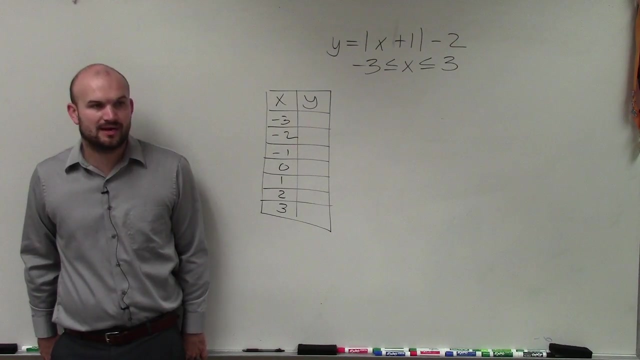 So I'm going to go negative 3, negative 2, negative 1, 0,, 1, 2, and 3.. Now for the first couple I'll do, and then I'll start doing them, and not in my head, but I'll kind of talk them out loud. 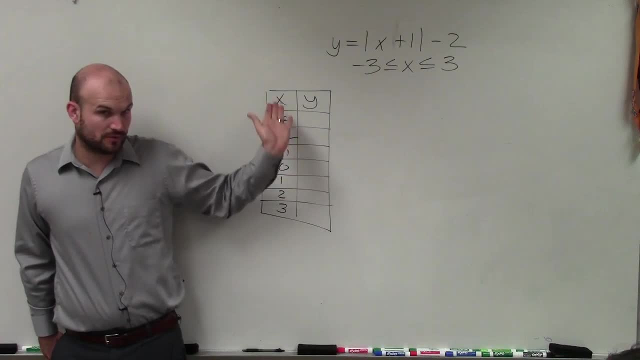 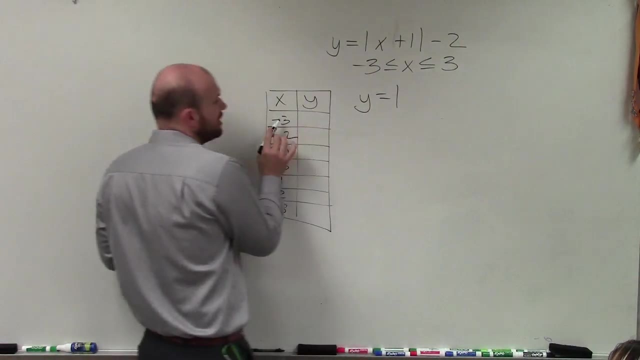 So to find the y values, so we give in our x values. These are what we call our arbitrary x values. To find the y values, all we're simply going to do is take our equation and plug in our value for x, or plug in our value in for x. 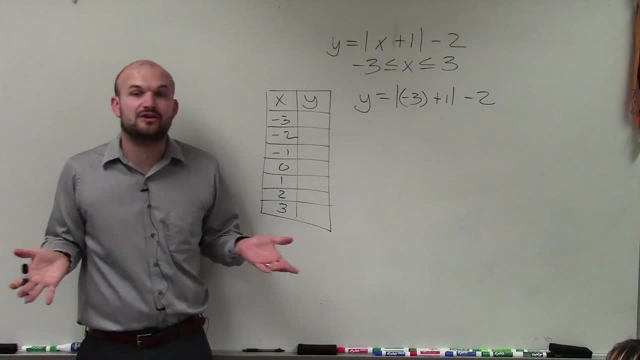 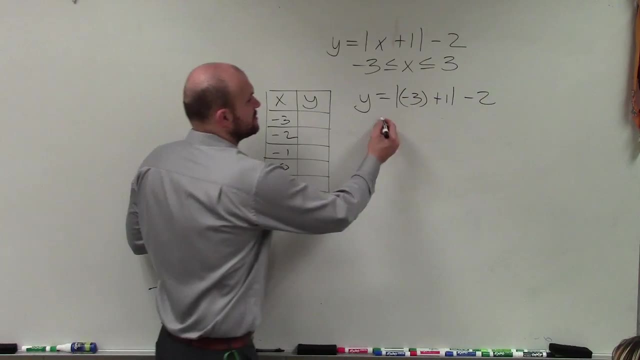 Now we haven't talked too much about absolute value functions, so just remember: absolute value represents the absolute distance, so it's always going to be positive. So I have negative 3 plus 1 is negative 2, so that equals the absolute value of negative 2 minus 2.. 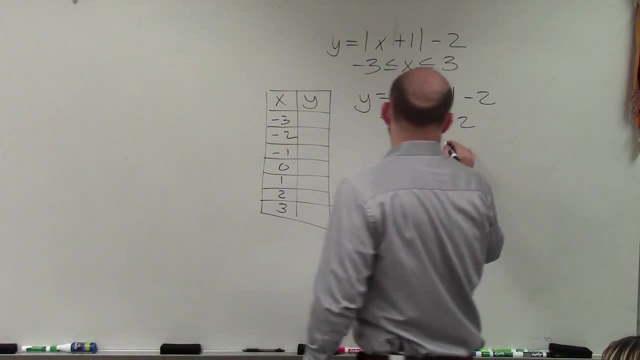 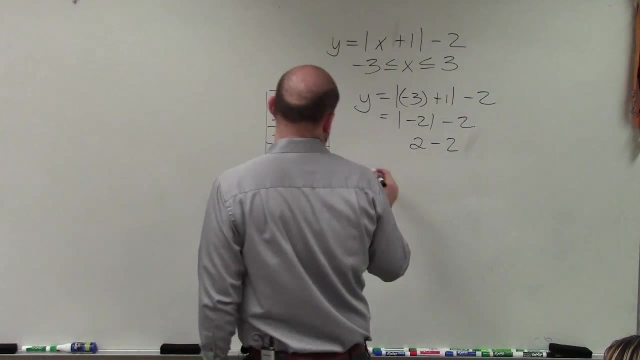 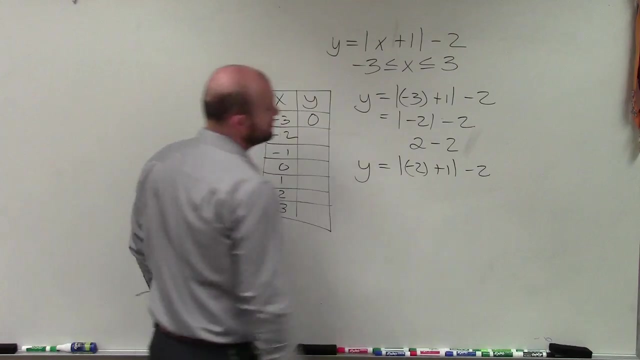 Well, the absolute value of negative 2 is going to be positive, So I have positive: 2 minus 2 equals 0. Then I'll do the next one: negative 2 plus 1, absolute value minus 2.. 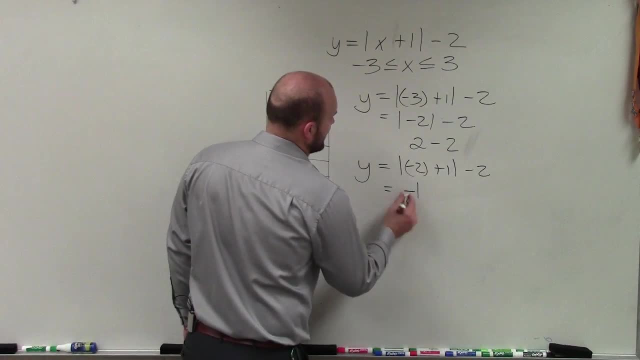 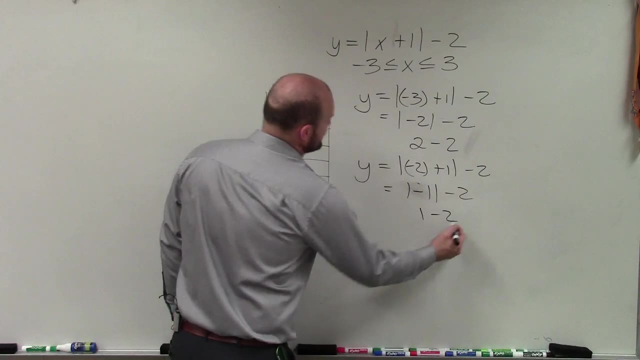 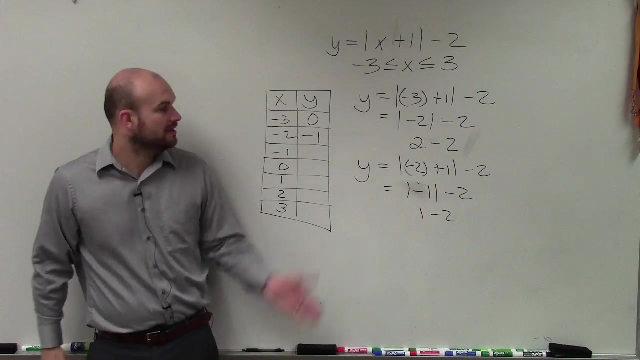 Negative 2 plus 1 is going to equal to absolute value of negative: 1 minus 2.. So absolute value of negative 1 is 1 minus 2 is going to equal negative 1.. Does everybody follow me so far? Okay, so now I'm just going to kind of do these in my head to finish the rest of the problem. 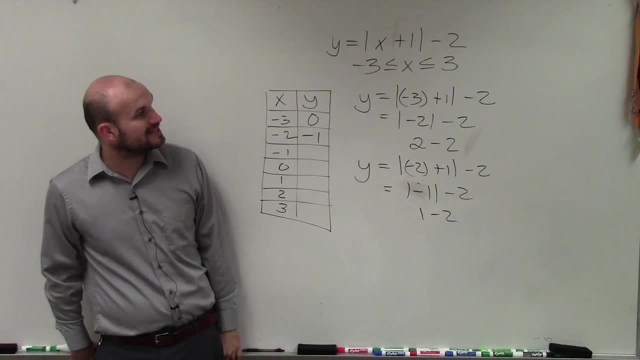 Negative 1, so I plug in negative 1 in for x. Negative 1 plus 1 is 0. Absolute value of 0 is 0 minus 2 is negative 2.. If I plug in 0, 0 plus 1 is 1.. 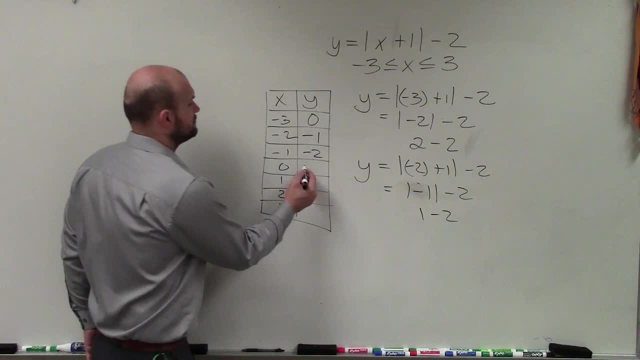 Absolute value of 1 is 1.. 1 minus 2 is negative, 1.. If I plug in 1,, 1 plus 1 is 2.. Absolute value of 2 is 2.. 2 minus 2 is 0.. 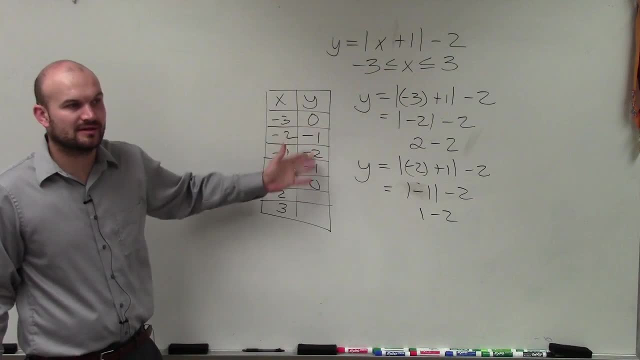 And hopefully you guys kind of see that. See, there's a little bit of a pattern here. They're kind of the same on both sides of that. 2, right, So let's do 2.. 2 plus 1 is 3..